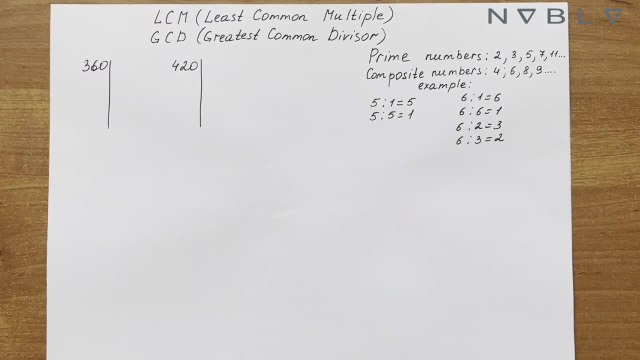 Now I will explain to you how to find the greatest common divisor and least common multiple of two numbers. Let's take, for example, two numbers: 360 and 420.. In order to find the LCM and GCD, you need to write both numbers into prime. 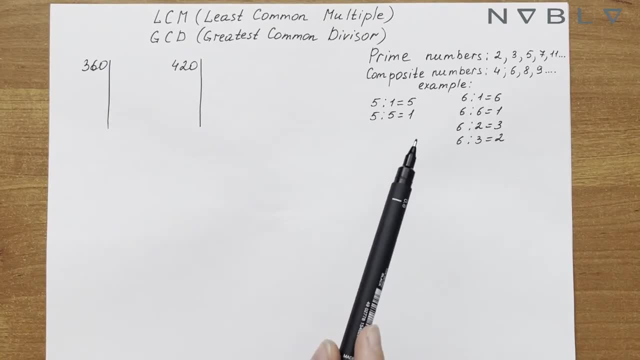 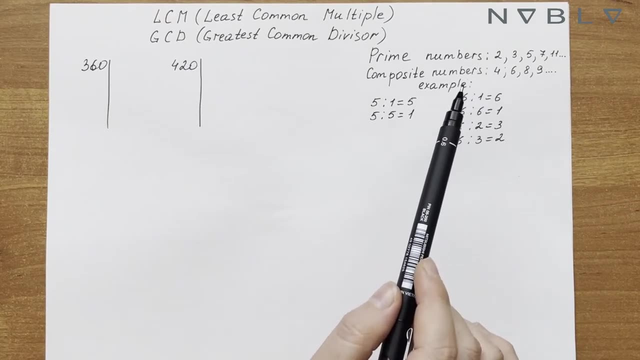 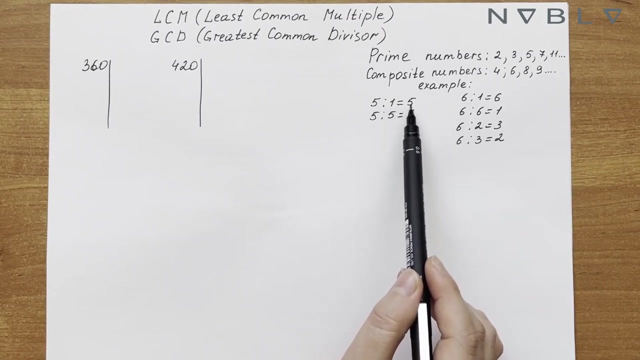 factors. Prime number is number, for example 5.. Prime number has only two factors: 1 and itself. 5 divided by 1 is 5, and 5 divided by 5 is 1.. 6: it's a composite number, because 6 has more than. 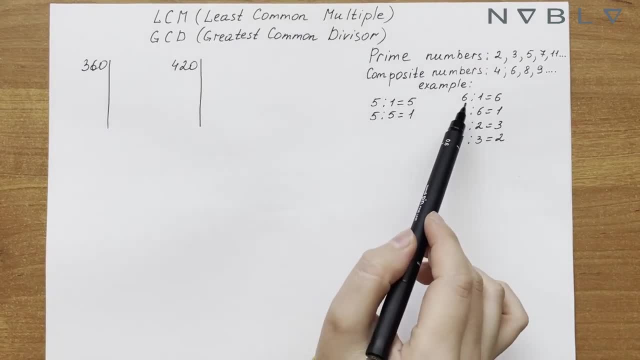 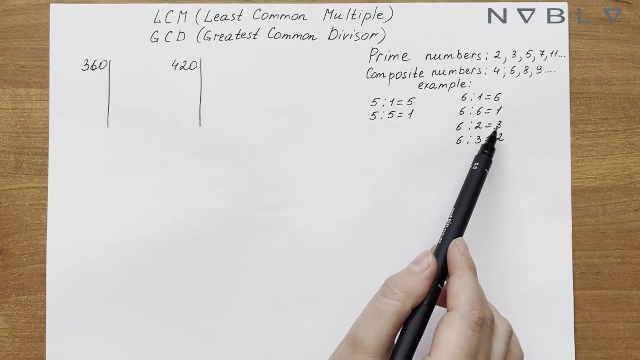 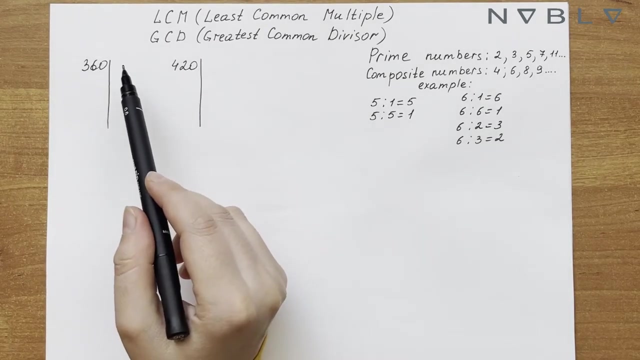 2 factors. Also, 6 divided by 1 is 6.. 6 divided by 6 is 1 and 6 divided by 2 is 3 and 6 divided by 3 is 2.. We write down the number line on the right side. We can. 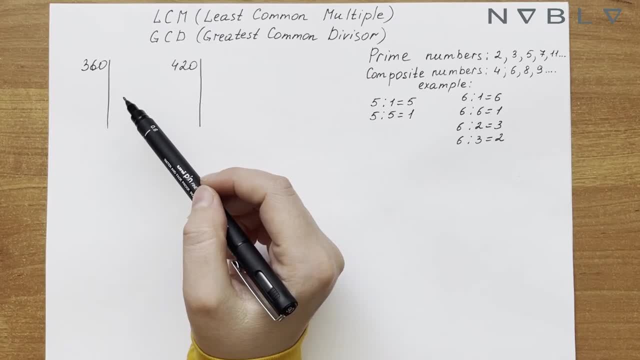 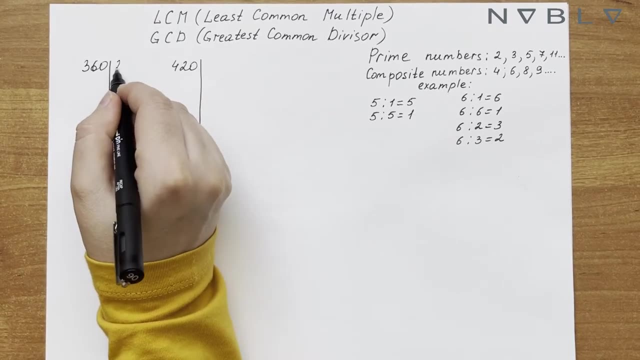 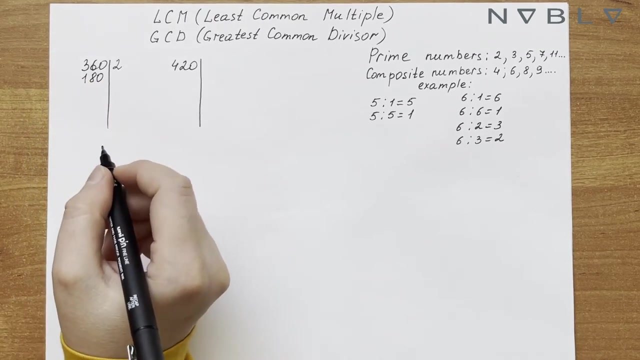 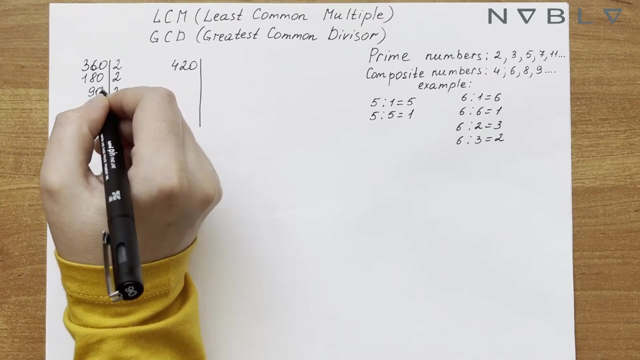 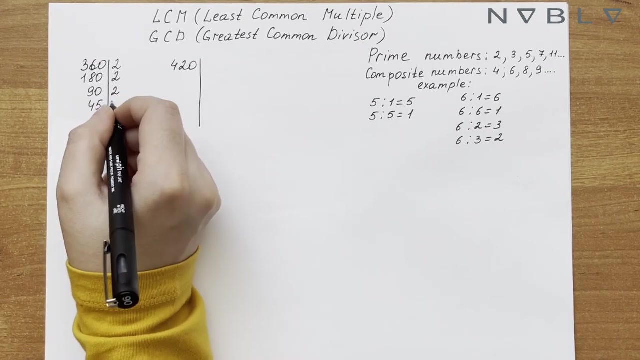 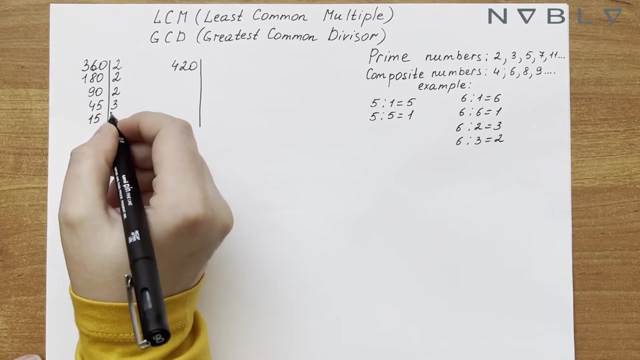 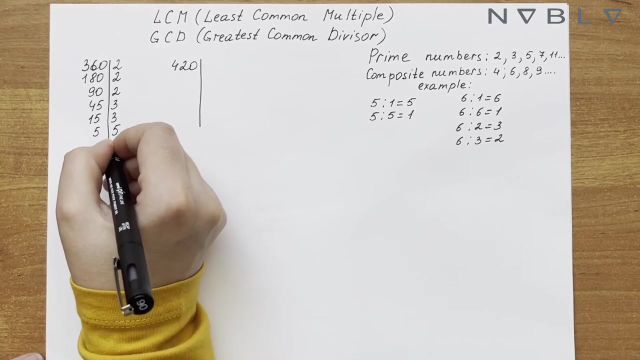 write down only prime divisors, and always the smallest. 360 divided by 2. There will be 180.. 180 divided by 2 is 90.. It will be 45. Here we divide by 3.. 45 divided by 3 is 15.. 15 divided by 3 is 5.. 5 divided by itself is 1.. When we got 1,, 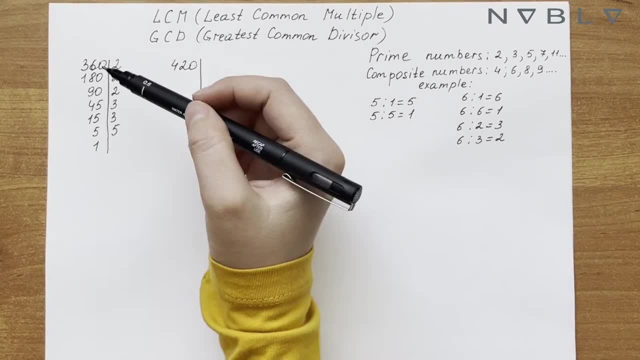 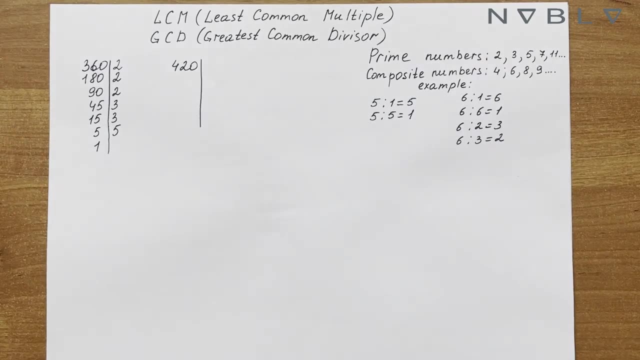 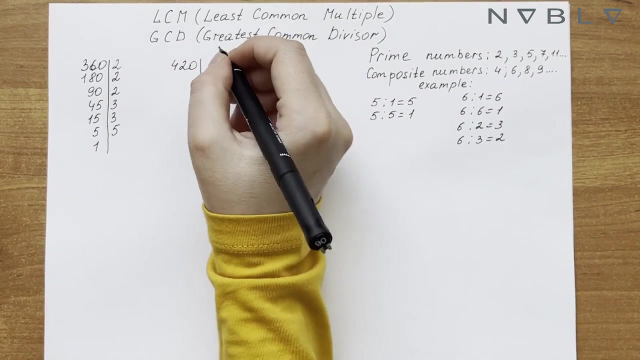 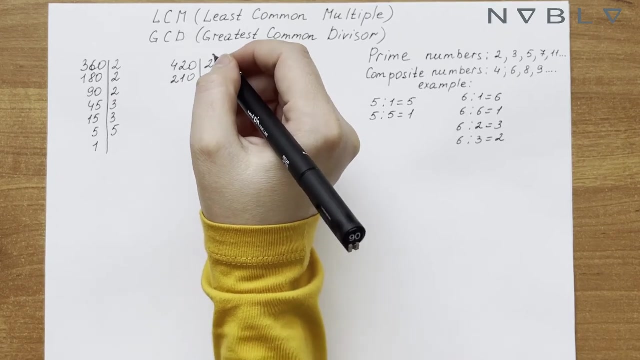 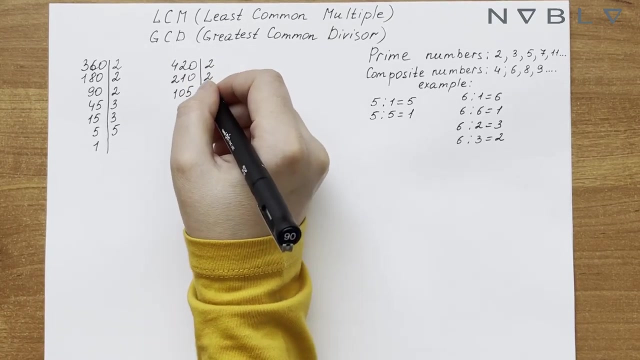 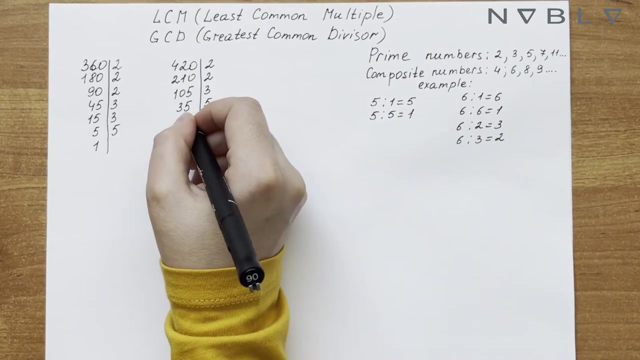 that's the end of the division. All numbers on the right side are prime divisors. We do the same operation with the second number: 420 divided by 2 is 210.. Again, by 2 is 105.. 3 is 35.. 35 divided by 5 is 7.. 7 divided by 7.